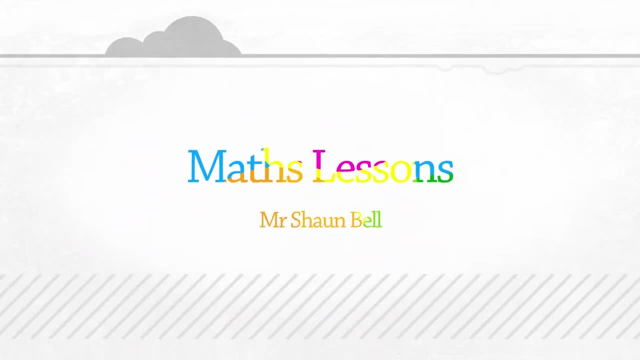 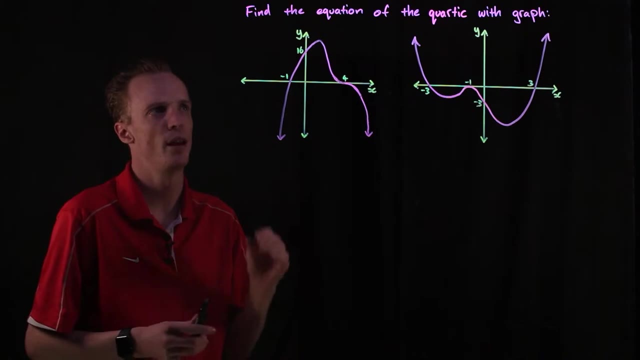 So what I want to quickly overview here is how we actually continue on and start finding equations for quartics. So what we can see here is we've got a couple of quartics with the axes intercepts given to us and what the axes intercepts tell. 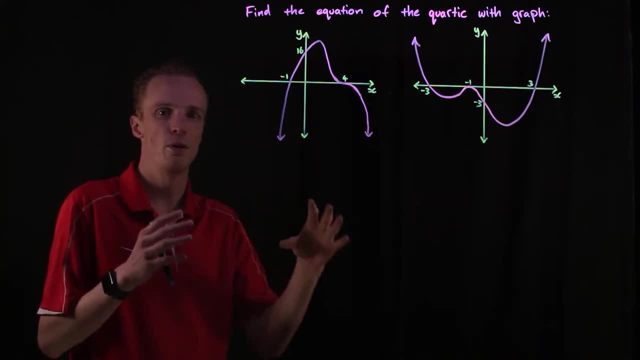 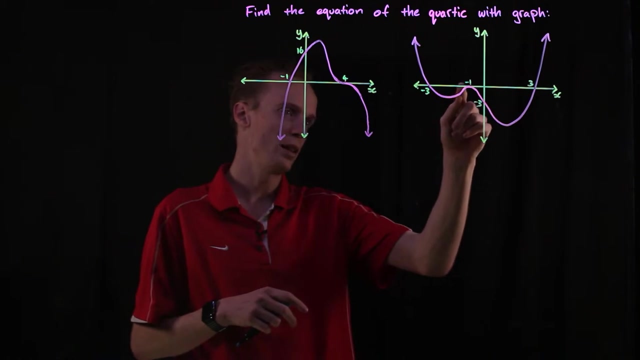 us particularly the x-axis is the type of root that we might have which each of these quartics. So, for example, when it cuts through, here we've just got a linear factor- When it has this stationary point of inflection, we've got a cubic linear factor where, if it just touches the x-axis, like we've got here, 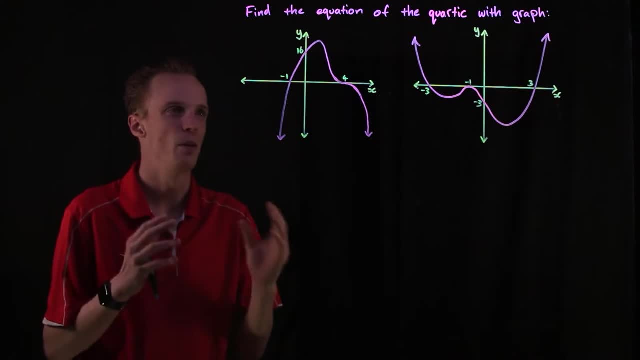 what we've got is a repeated linear factor. Now, one factor that isn't part of these two graphs is if we've got that real flat bottom one or that flat top one where we've got that quadruple linear factor that we've got to just 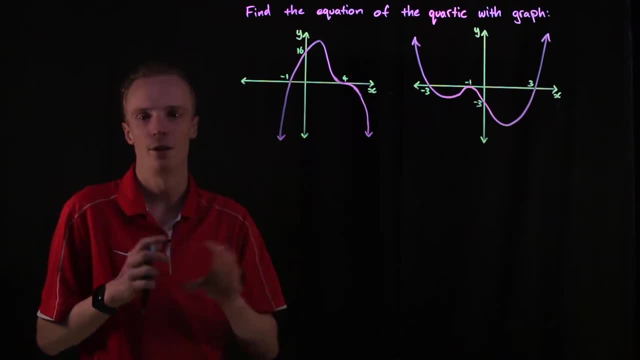 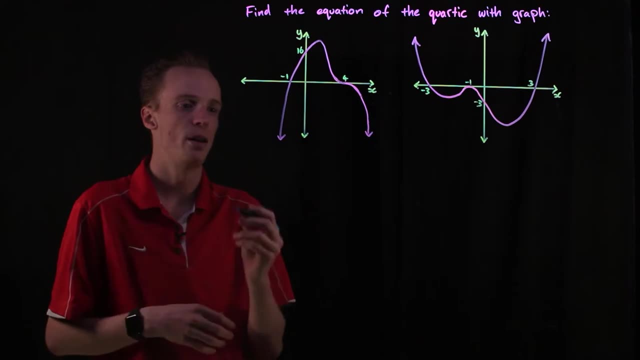 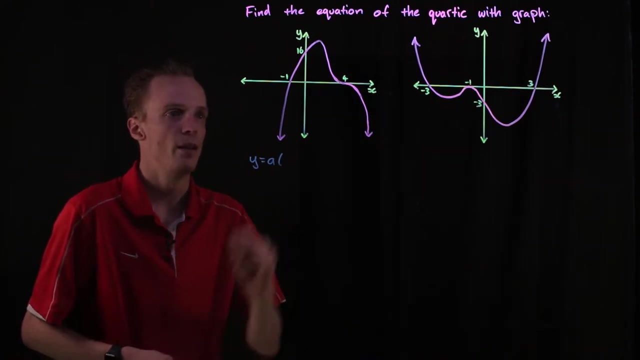 keep in mind you might come across Now. with each of these, you follow a similar process that we did with our quadratics and our cubics when we're finding them, in that we start by representing just a general cubic polynomial where we include the factors that we've got Now, because this 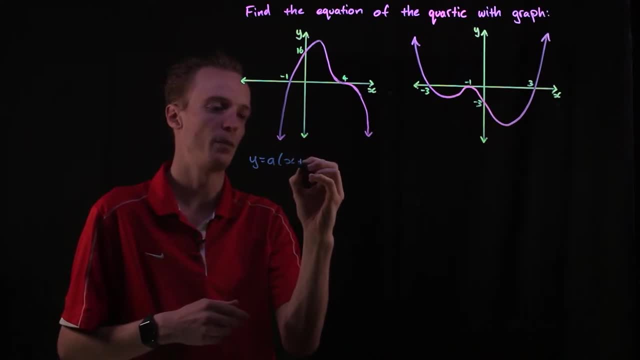 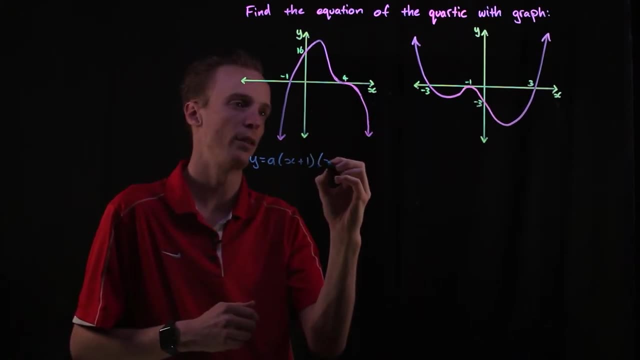 is cutting at negative one. the first factor that we've got is going to be x plus one. just the opposite sign of what we had here and because we've got this stationary point of inflection at this other point. so there's x minus 4 here. 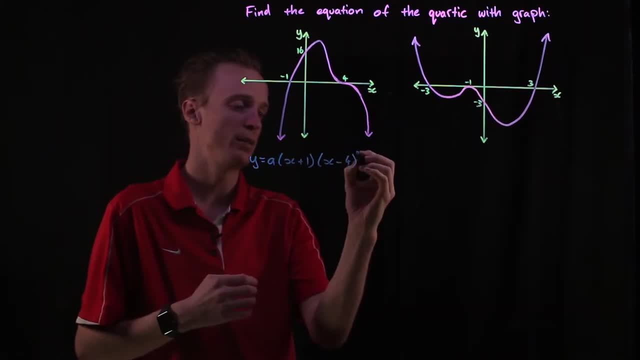 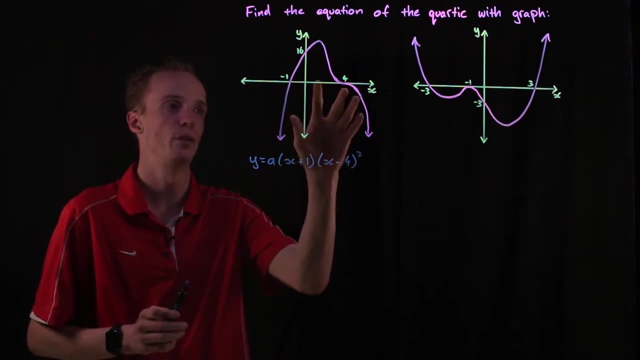 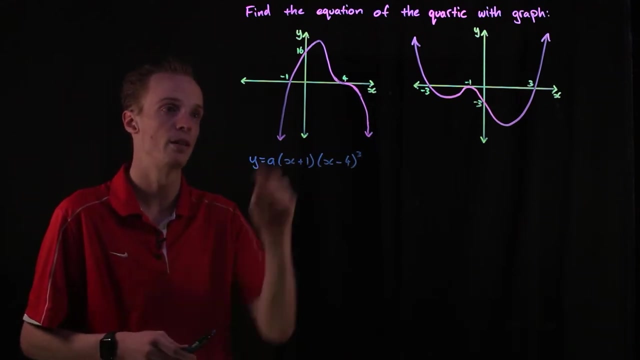 what that stationary point of inflection indicates is: this is going to be a cube linear factor here And now. what we've got is this general function for all cubic polynomials that cut through at those two points in that manner. But I need to define this value of a, So to do that, I need to substitute another point, that's: 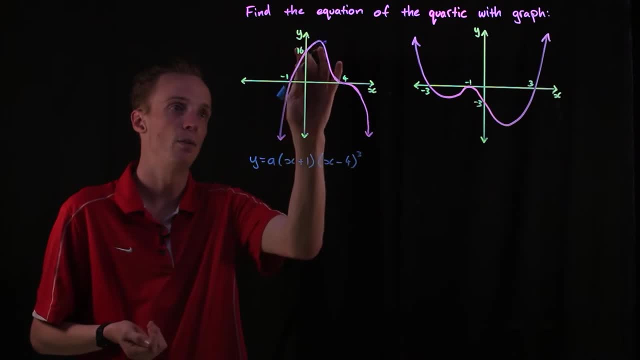 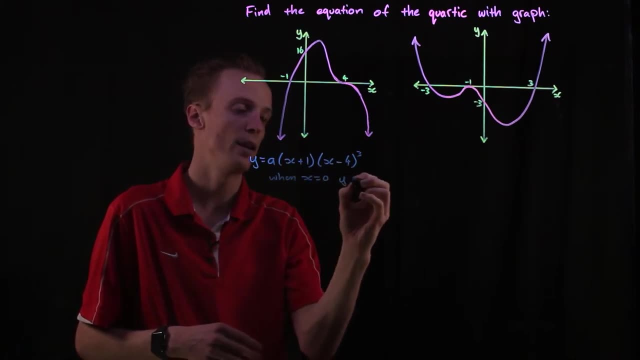 not one of the roots I've already used. Now it's given us the y-intercept here. So what that tells us is: when x is equal to 0, our y is equal to 16.. So that's the point that I can substitute in. 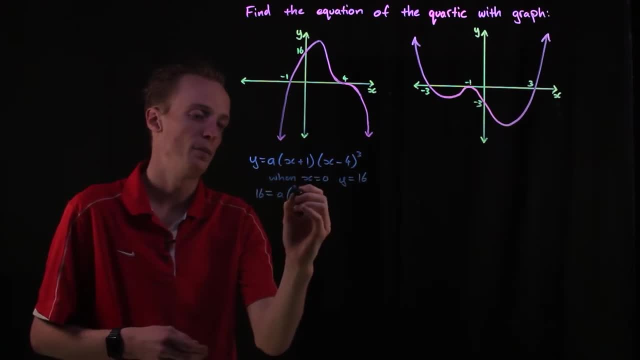 So 16 will equal. a 0 plus 1 is going to be 1.. 0 take 4 is negative 4 and that will be cubed here. So when I expand that out, this will be negative 4 cubes negative 64.. So it'll be negative 64. 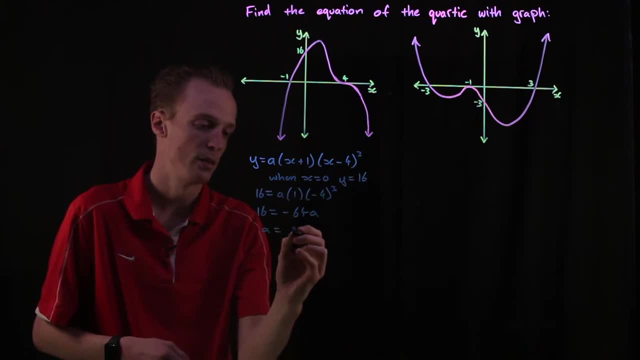 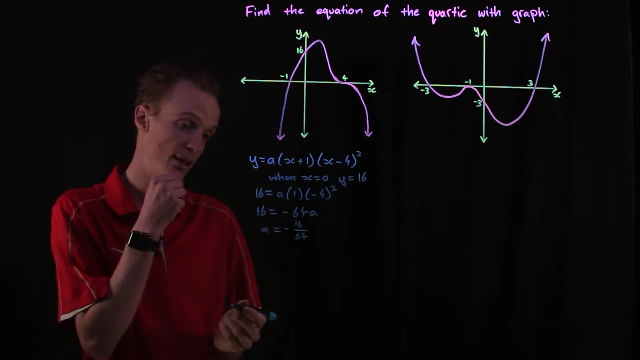 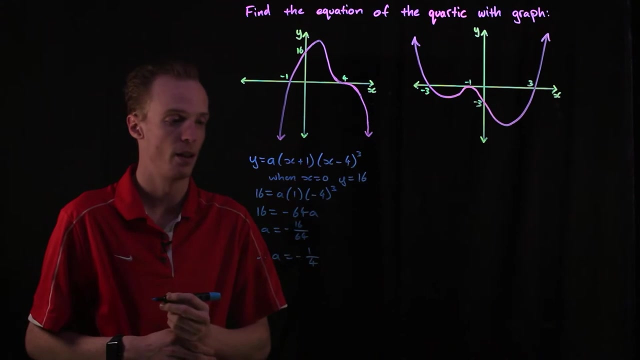 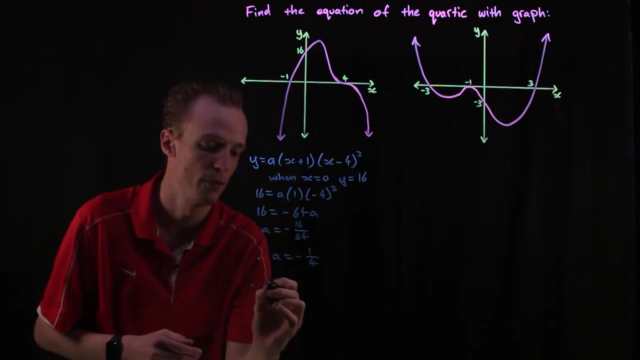 a here. So my a is going to be negative 16 over 64, which means that 16 divides into them both. So therefore my a is going to be equal to negative 1 over 4, like that. So to find the final equation here, I just substitute my a value back into here. So what that means for my final. 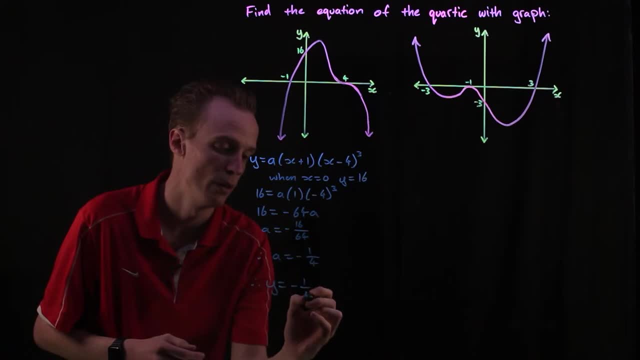 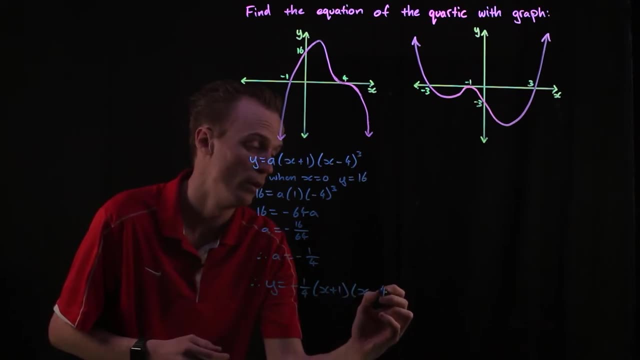 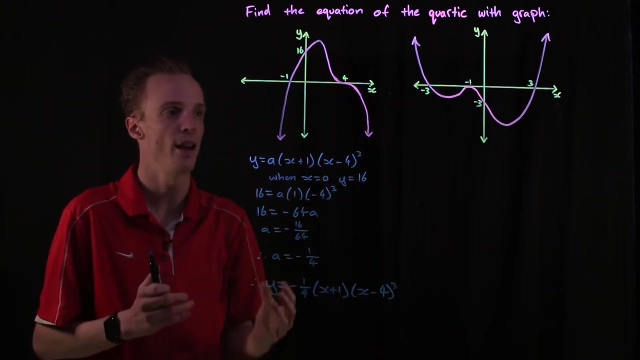 equation is: my y is equal to negative, 1 quarter x plus 1 and x minus 4 all cubed. Now, if I think about it for a moment, my a should be negative because I've got this overall concave. Now imagine this: So you get a center of axis of x�� stands out from the r? sine line and this: 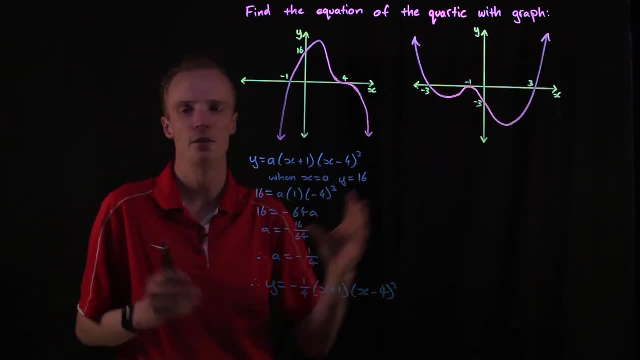 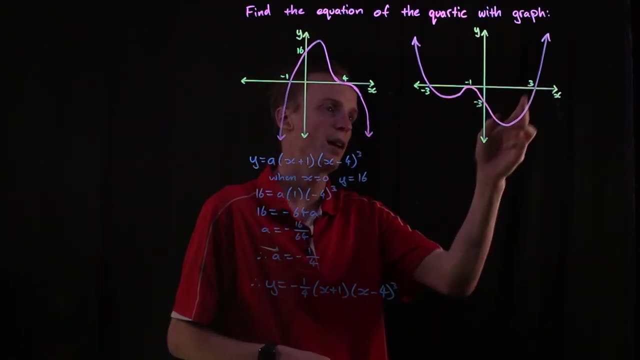 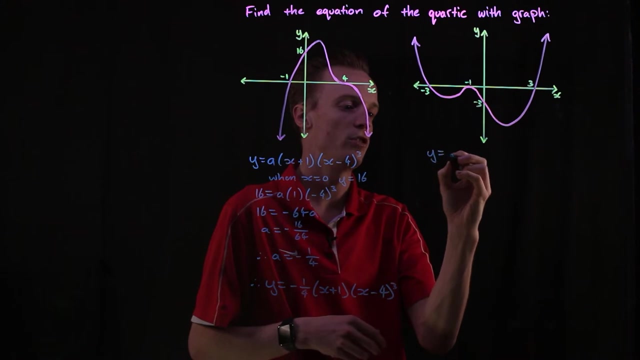 top invented legs and this bottom So that hills up. this is critic, hago. So you're going to solve this. So all of your values to be at the bottom of your collaborative films. em toff, it's going to cut here and cut. 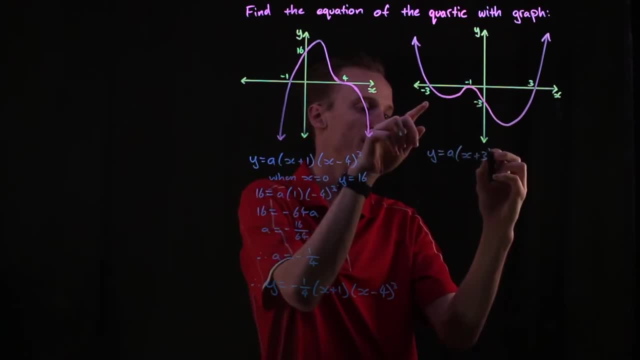 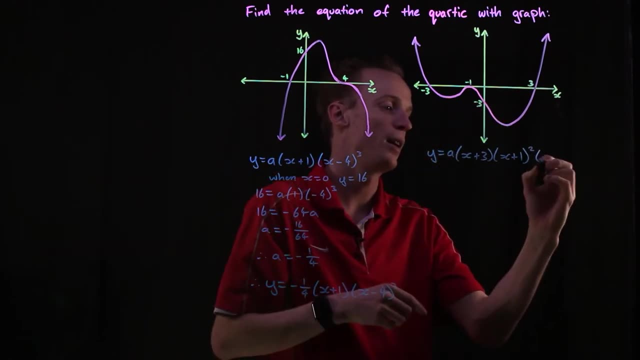 here's so just going to be linear factors and touches his. that's going to be a repeated root. So when I look at my function in just that general form, I'm going to have this x plus 3 for this root- that'll be a squared- and then my x take three for the final root over there. and now I need to. 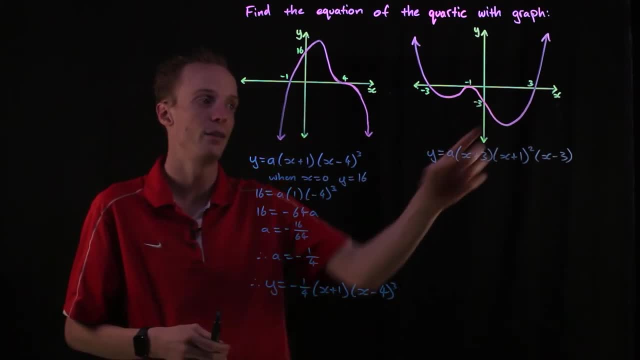 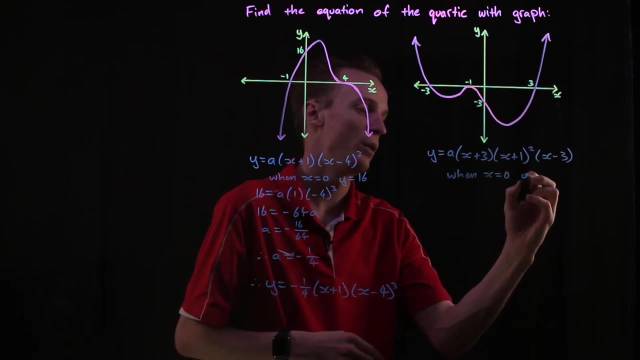 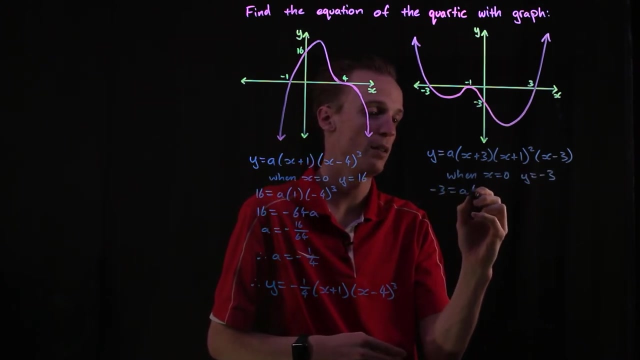 substitute a point in again. so the point that I'm going to substitute is the y in set, because that's what's given to us. so when my x is equal to zero, my y is equal to negative three here. so my y of negative three should equal a zero plus three is three. zero plus one is one and zero take three is. 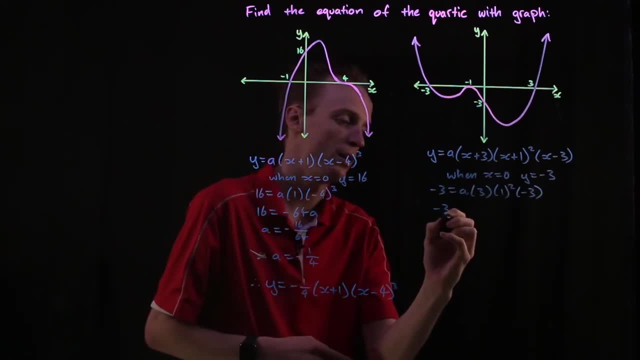 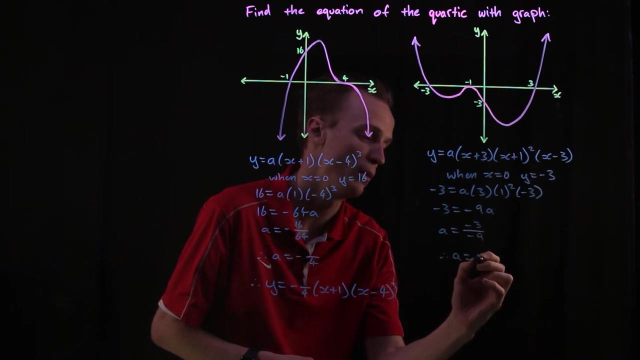 negative three. so when I expand this out now three times, one is three, it'll be negative nine, a like that. so a will be negative three over negative nine, which will just simplify to a positive one third like that. so now I've found my a. I just substitute that back into up here. so my function here is: y equals one third.